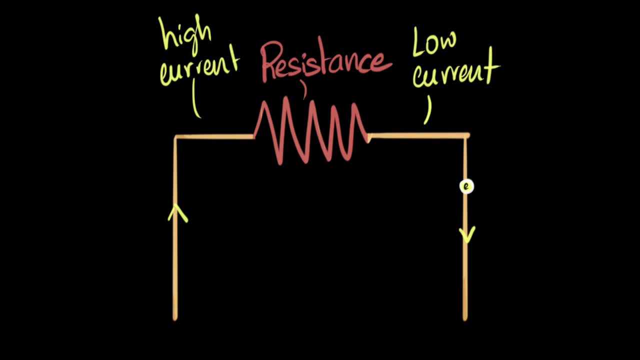 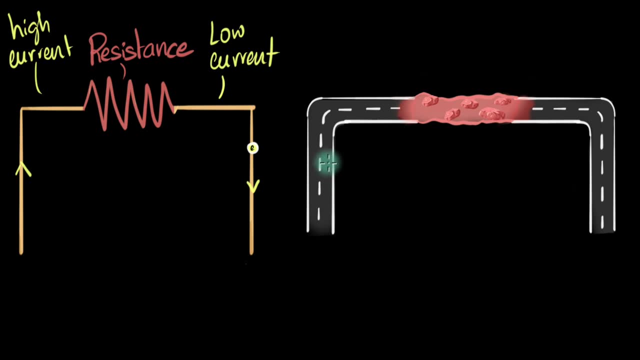 model to help me grasp this, because when you're learning things for the first time about circuits, you can't imagine circuits. So one of the models that I use- my teacher helped me model it was by thinking of it as a road and thinking of resistors as obstructions in the road. So we can imagine. 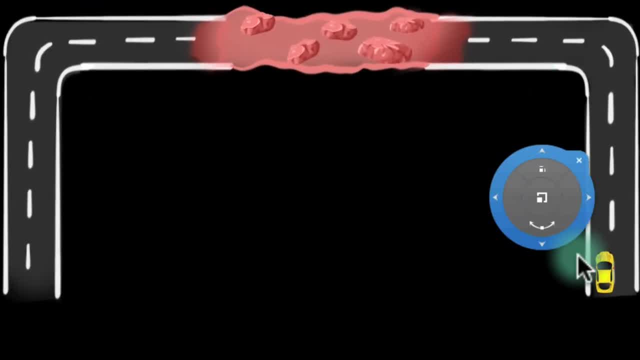 that there is a car. Where's the car? Okay, here's the car. So let's say there's a car And let's say we give a kick to this car. Imagine this is a toy car. It doesn't have any engine. let's say You 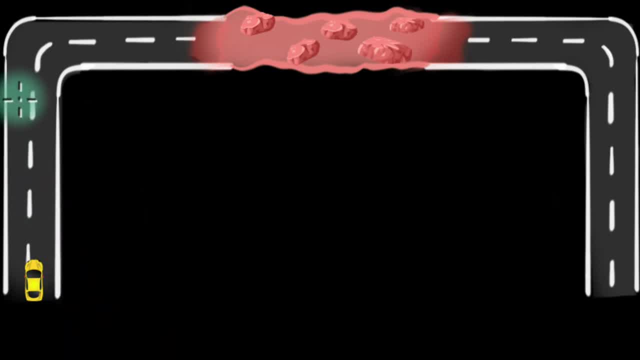 give a kick to this car over here, And then something very similar would happen, right? So if there is no obstruction, very smooth highway, the car would go very quickly over here, very fast. And then there is an obstruction, This is where the car would slow down. Remember, there are no. 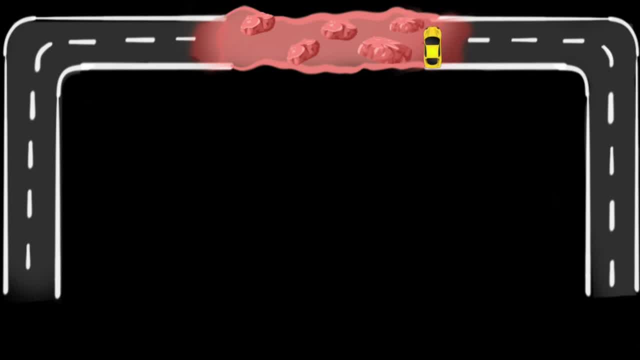 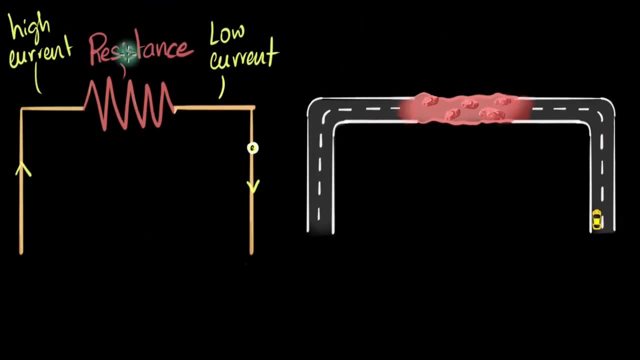 engines in the car, it would slow down, And if it doesn't stop already it would come out very slowly from this side. So it kind of makes sense. This makes sense. So one side should have high current, the other side should have low current, the charges should slow down. But 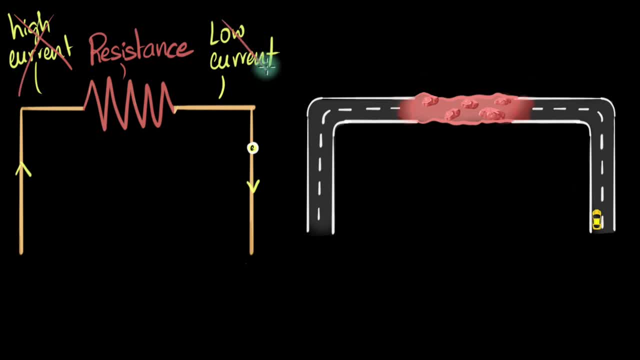 guess what That's wrong. It turns out that's not true, It turns out. when you learn about these circuits, you learn that in this circuit, if you take a very simple circuit, there are no branches and everything. then the current is the same everywhere. we get the same current And my 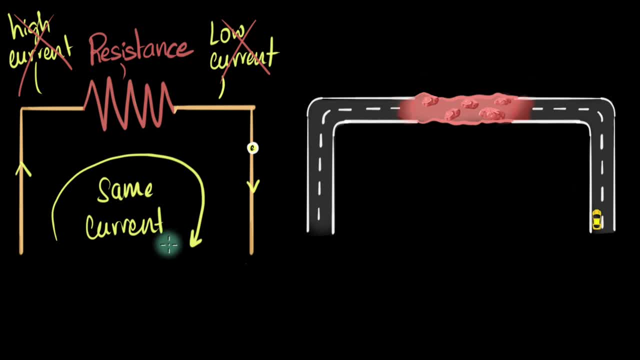 question was: why or how does that make any sense? Well, it took me a while, But then I realized the biggest mistake we are making over here is: you're assuming there's only one electron in this entire circuit there, And that's wrong. There are electrons everywhere. How does that help us? Well, 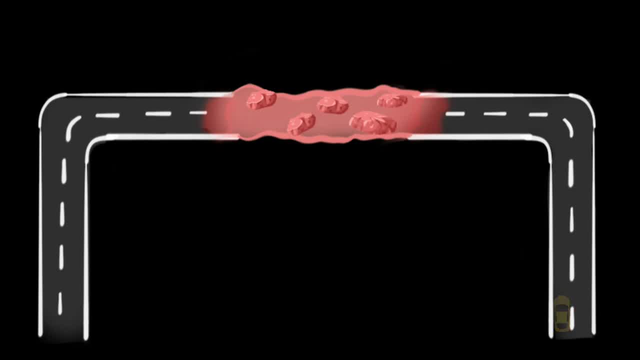 let's come back over here. Instead of imagining there's one car, which is wrong, we have to imagine there are cars everywhere. So there are cars everywhere. Imagine there is no space for them to go. It's like completely jam packed. Now think about this: Although the cars over here are going, 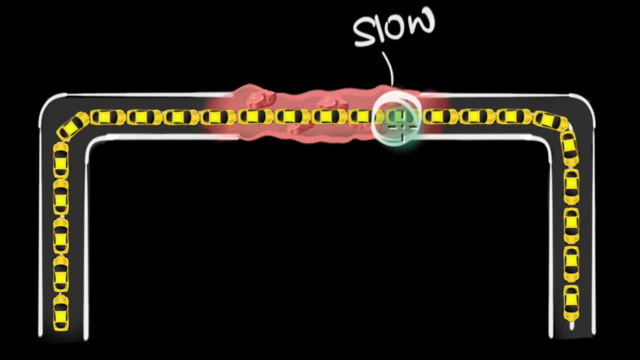 super slow because of all the obstruction. the car behind it can't go anywhere. It can't go anywhere Faster. the car behind that can't go any faster because there is no room for it to go any faster. Similarly, the car over here: Yes, there is no obstruction, But hey, it has no room for it to go.